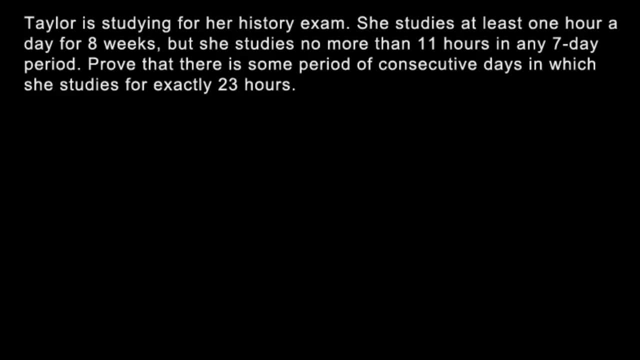 is a pigeonhole problem. It's not too obvious to see exactly why, but the concept of having a period of days where you have to fit in a certain number of hours, like the concept of fitting in something, should remind you of the pigeonhole principle. So to start this off, 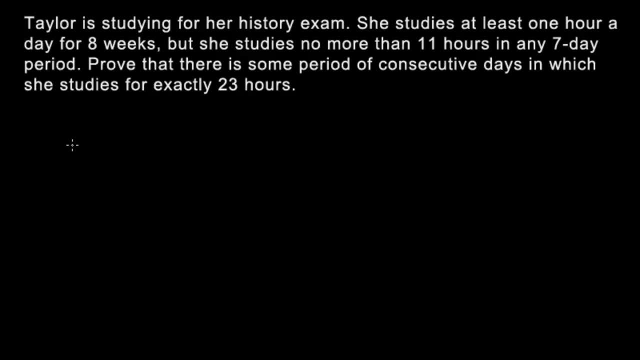 I'm going to show you what this problem really means. You have 56 consecutive days, eight weeks, because it's 56 days. During 56 days, you study a minimum of one hour each day, But in any period of seven days you study no more than 11 hours. So you study no more. 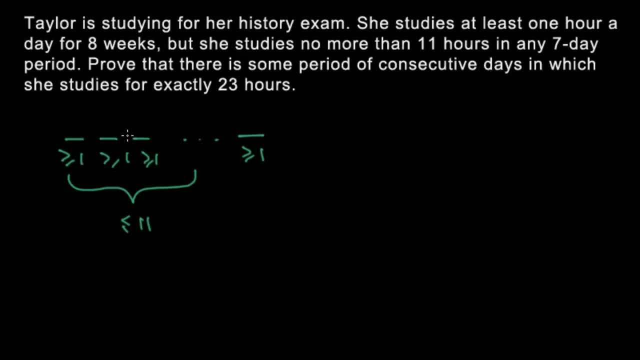 than 11 hours. So the questions asking prove that there is a certain number of days where you study exactly 23 hours. So say that this is n days, then you study exactly 23 hours. So this is what the problem is asking us right now. I'm going to introduce the notation of si. 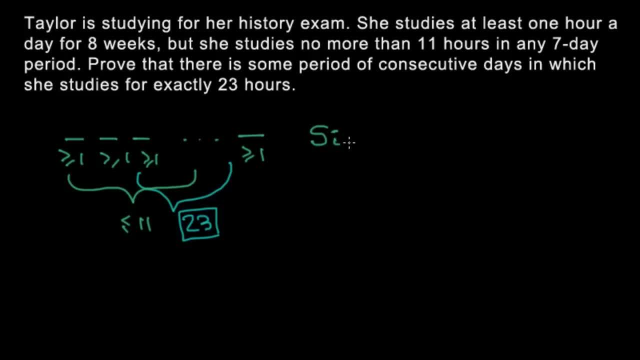 let si be the number, the number of hours Taylor studies until the until the i-th day. I used s because it's the sum. For example, just give you an example. Say that she studied one hour in the first day, Three hours in the second day, two hours in the third day, one hour in the fourth day. 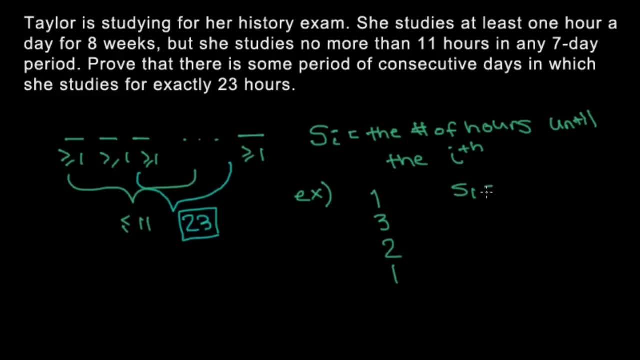 And the corresponding si would be: s1 would be one hour, because she's only studied one hour in the first day. s2 would be one plus three, which is four. s3 would be one plus three plus two, which is six, and so on. So that's what si is, And then what we're trying to find is: 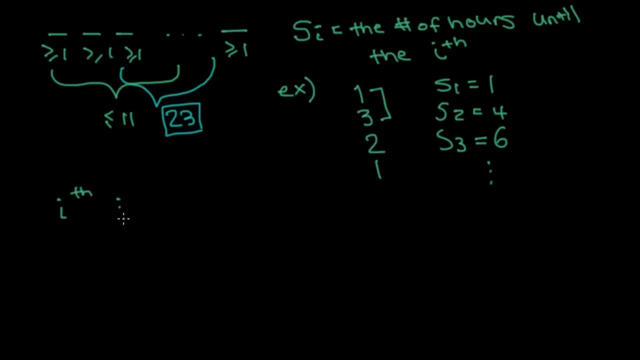 for some i-th and j-th day, where let's just say j is bigger than i, where this is satisfied, there exists sj minus si, where it is exactly 23.. And this is because, during the interval of 56 days, 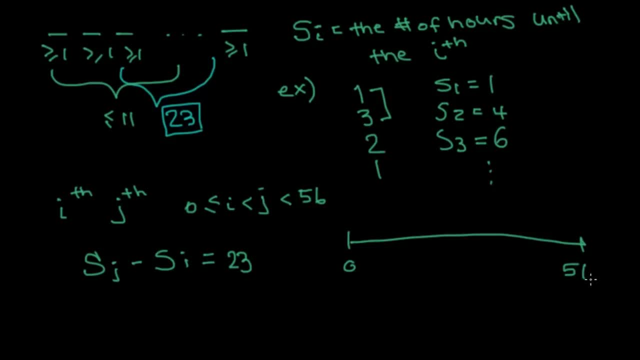 where this is zero and this is 56, and i is right here and j is right here- the number of hours she studied during this period is sj, And also the number of hours she studied this period, during this period, is si. 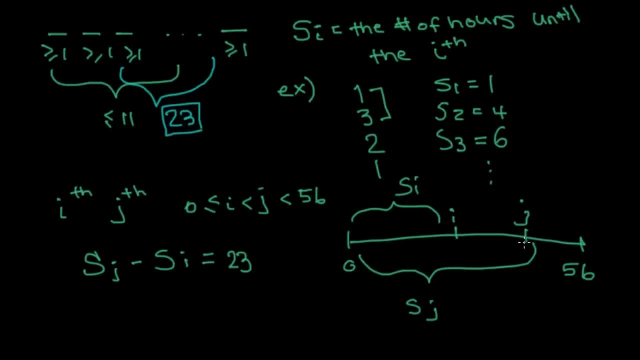 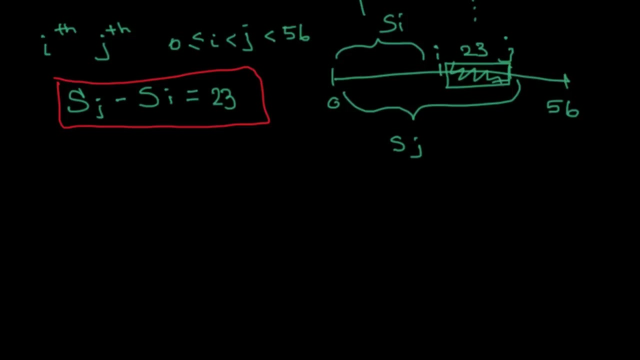 We need to show that right here. sj minus si, this is exactly 23.. So this is what we're trying to prove. We also know that there are eight weeks and she can only study 11 hours per seven days. So in total, during the 56 days, she can study a maximum of 88 hours in total. 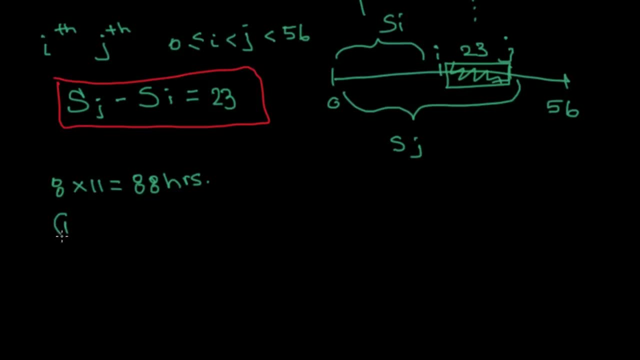 So this inequality, let's just say number one- we know that minimum of one hour on the first day, s1,, s2,, all the way up to s56, is less than or equal to 88 hours. We're going to create another one where we add 23 hours to each term. 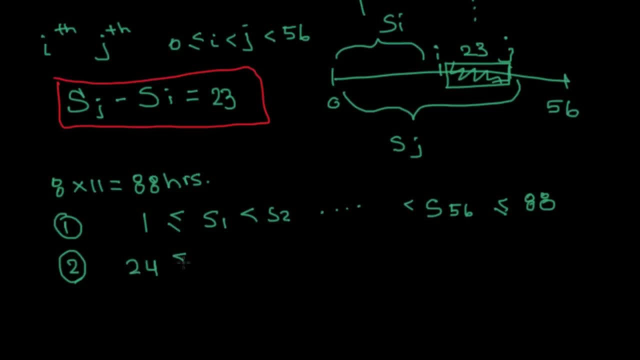 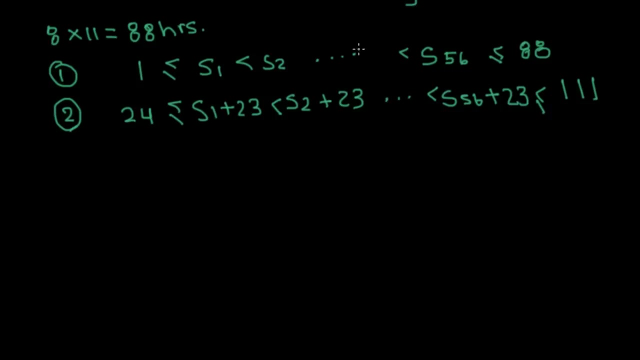 So this becomes a minimum of 24 hours: s1 plus 23,. s2 plus 23.. All the way up to s56 plus 23 is less than or equal to 88 plus 23,, which is 111.. Now this is where we're going to use the Pigeonal Principle. 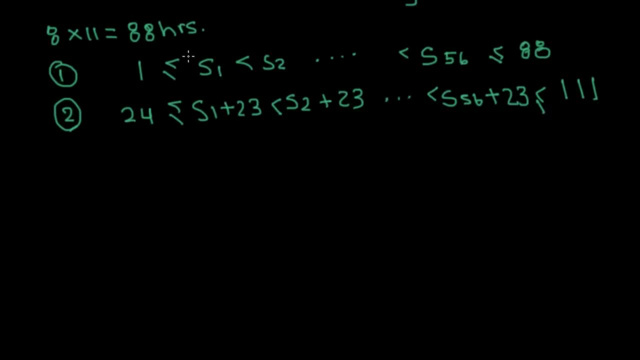 So, looking at this right here, we have a total number of 56 plus 56 terms, which is 112 terms. So this list right here: s1, s2,, all the way up to s56, and also s1 plus 23,, all the way up to s56 plus 23,. 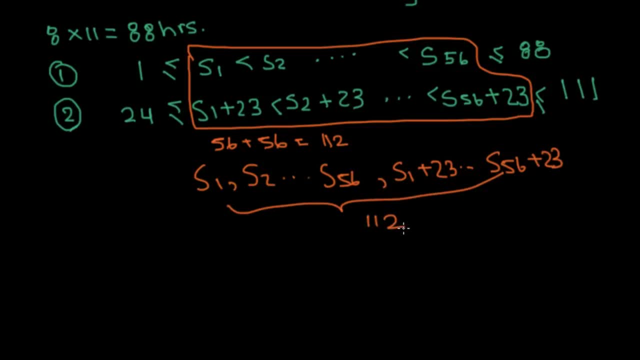 we have 112 of those. But looking at this- 124,, 88,, 111,- we know that this number right here is also between 1 and 111.. The Pigeonal Principle tells us that while there are 112 numbers and a range of 111 numbers,